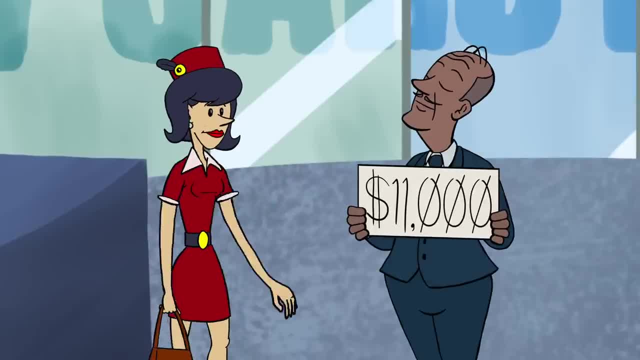 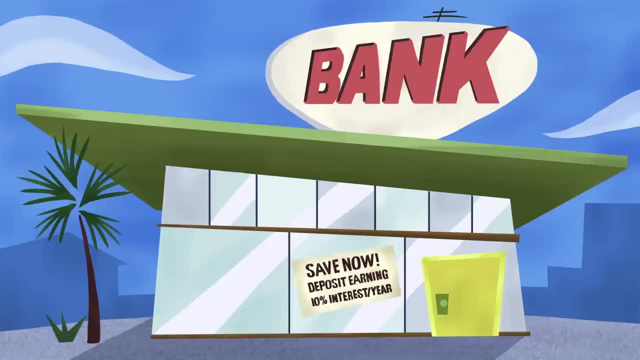 Yes, Sheila, that's a nice car. Oh, looks like Sheila is a little short, But wait, she has an idea. Sheila is a smart cookie. She knows that if she deposits the money for a year instead of buying the car today, she will earn interest. 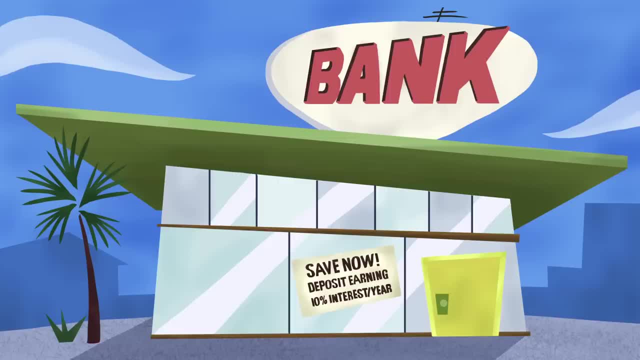 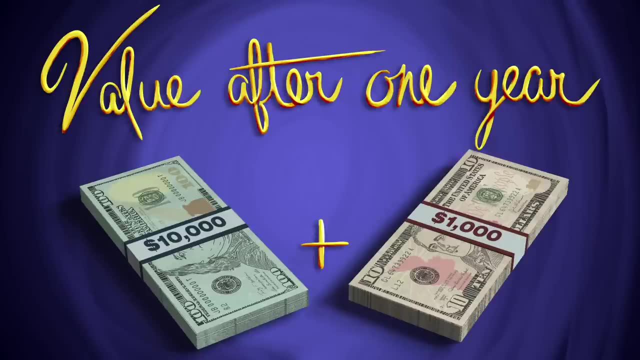 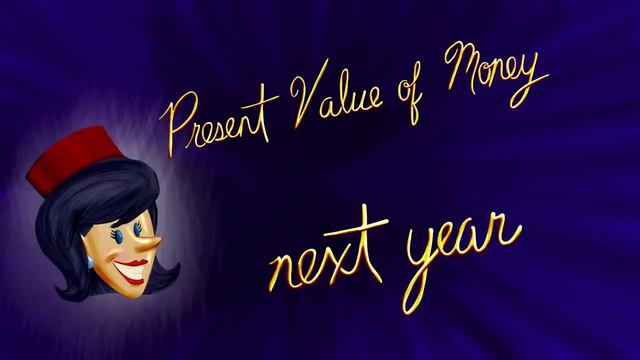 Then she'll be able to afford the car. Sheila knows that the value of her deposit one year from now will equal the money deposited today plus the interest earned. We call Sheila's money deposited today the present value and the value of Sheila's deposit next year. 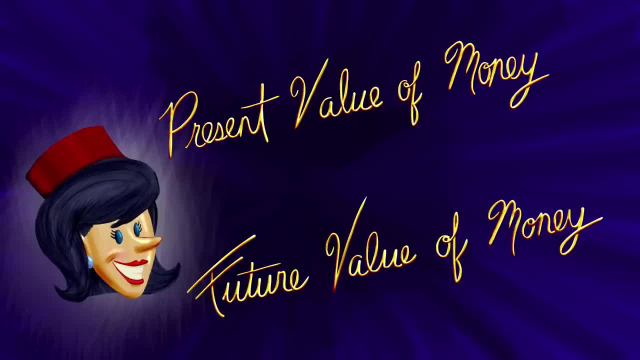 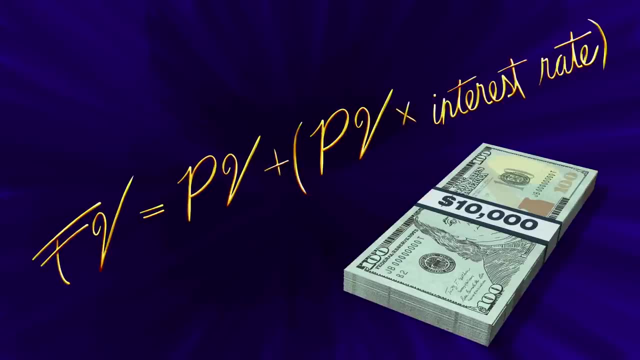 is the future value of money. What connects one to the other? The interest rate, also known as the time value of money. Now, with a little bit of rearranging, we can figure out the future value of Sheila's money with this equation. 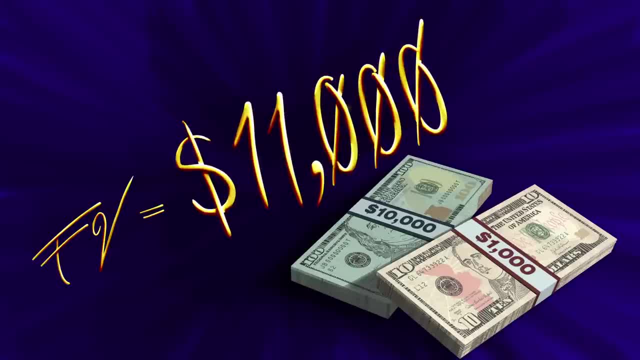 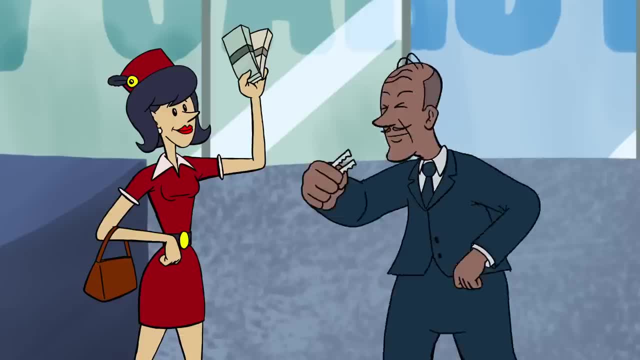 So in a year the future value will be $11,000.. Well, it's been a year and there's Sheila, with enough money to buy the car. Sheila really understands the future value of money. now I just hope she understands the speed limit. 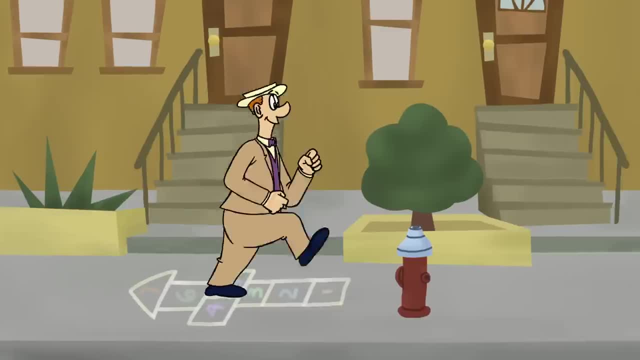 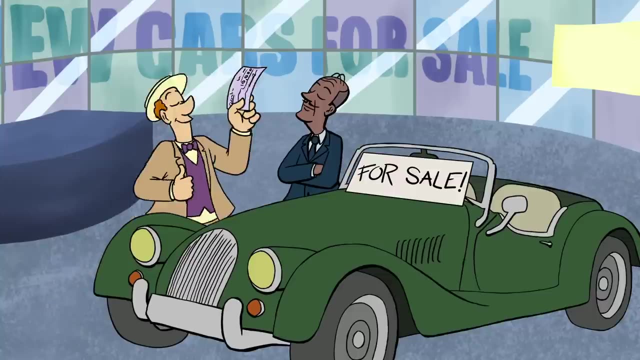 Now meet Timmy. He's also gotten his bonus. The money seems to be burning a hole in his pocket. Yes, Timmy, that's a nice car. That will surely impress people. Oh, looks like you're a little short. 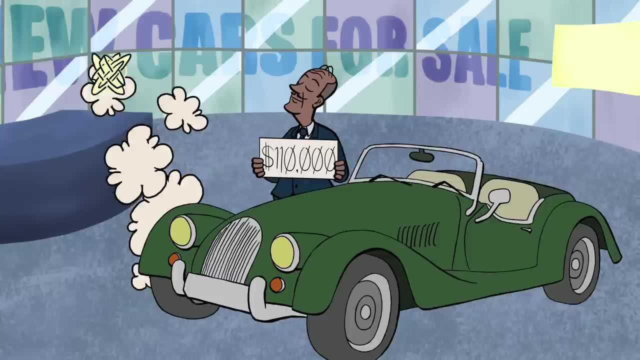 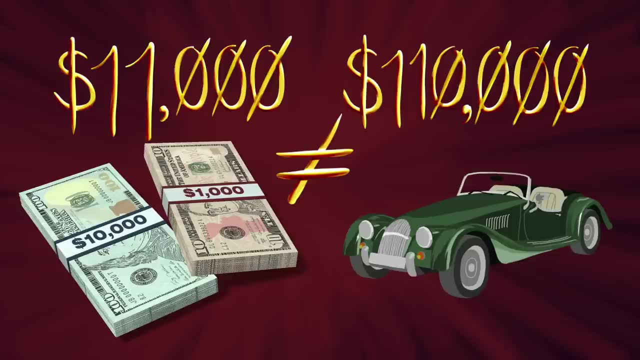 Maybe you can follow Sheila's example. You see, Timmy, just like Sheila, after the first year you'll have $11,000.. But, Timmy, that is still not enough to buy that fancy car. Why don't you leave the money deposited for another year? 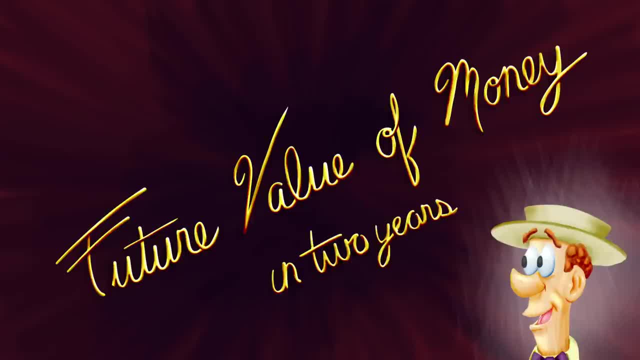 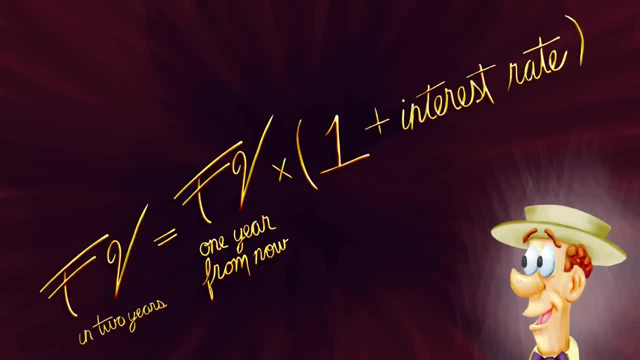 Let's see how your deposit would be doing in two years. With a little bit of rearranging, it becomes the value of your money next year times one plus the interest rate. We can then convert the future value one year from now to the present value times one plus the interest rate. 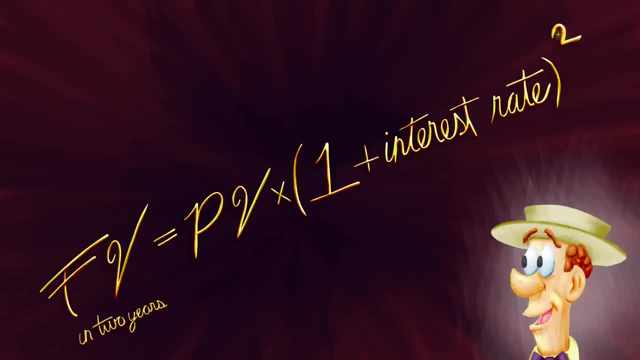 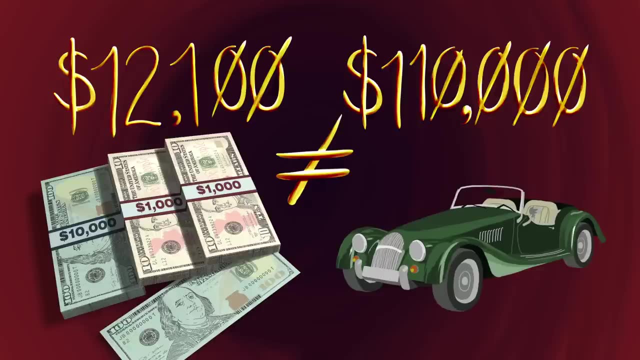 We can even simplify this further by just squaring the value of one plus the interest rate. Sorry, Timmy, you'll have more money after two years, but you still can't afford the car. I don't know how many more years you'll have to wait.